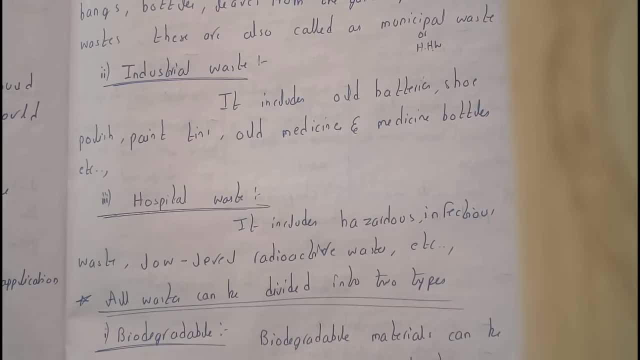 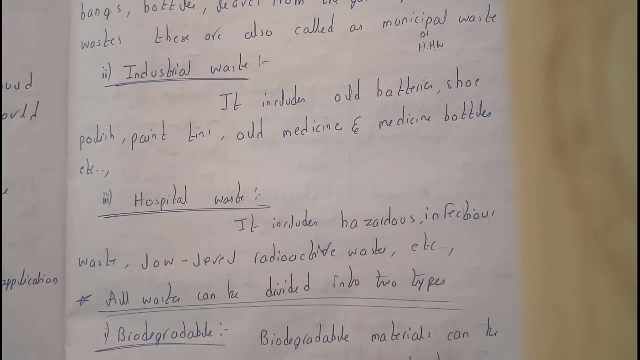 I hope everyone visited hospitals at least once, So there will be. medicines are made from different, different chemicals As those wastes. if there is a waste, if they are collecting wastes in a hospital, there may be expired medicines And many other chemicals. they are nothing but just chemicals. guys in hospital. 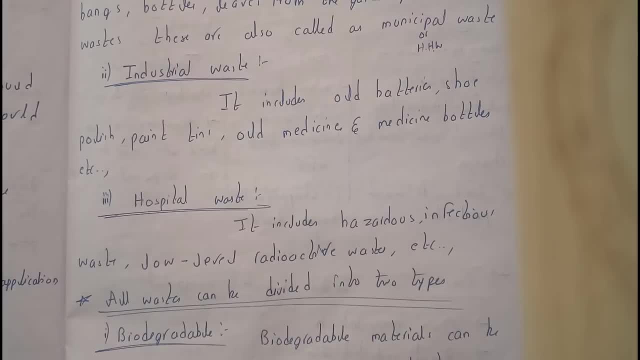 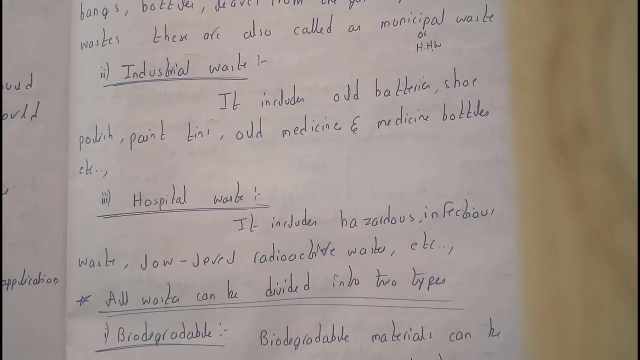 If you find any waste that is made up of chemical. So these are all the types of solid wastes around us. So these solid wastes can be few can be degraded and few cannot be degraded. Degraded means decomposed. Okay, We'll be going through it. 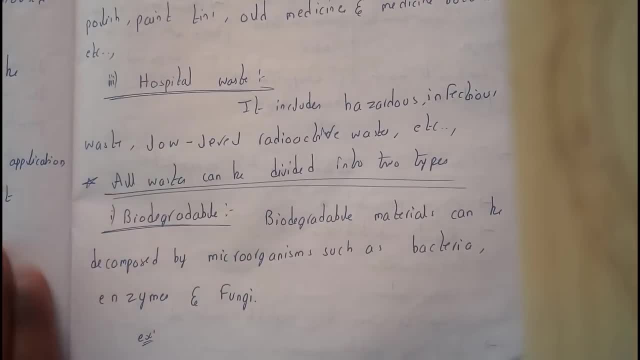 So all solid wastes are divided into two types, guys. One is biodegradable, Another one is non biodegradable. Okay, Biodegradable are nothing, but they can be decomposed by organisms such as bacteria, enzymes and fungi. Okay, biodegradable means which can be decomposed by microorganisms. 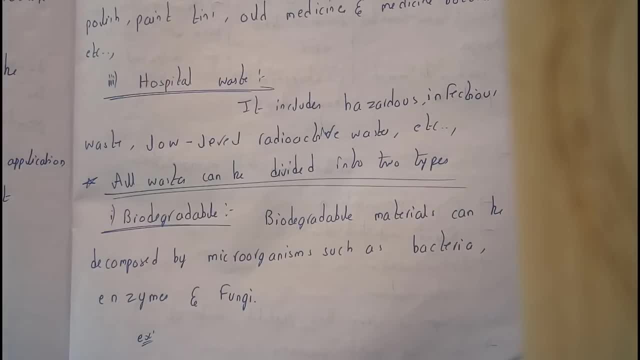 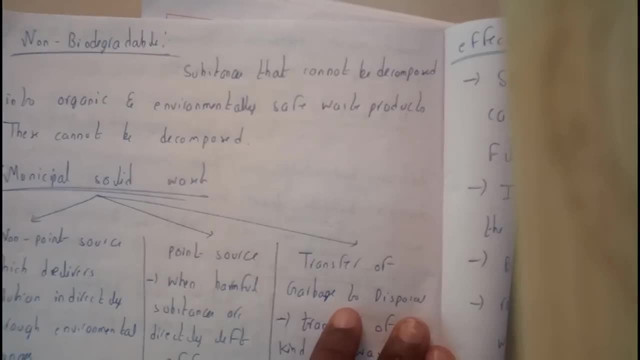 I hope everyone got a small idea, at least a small idea. Let's go through: non biodegradable. Non biodegradable substances are nothing, but they cannot be decomposed. That's it, by the environment. Okay, They cannot be decomposed. 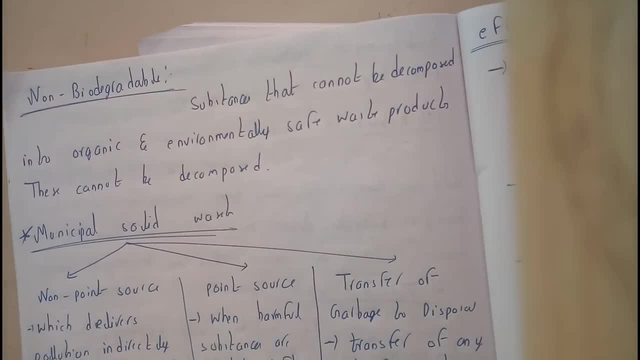 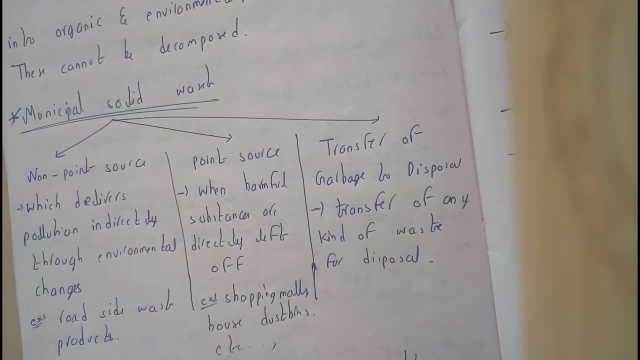 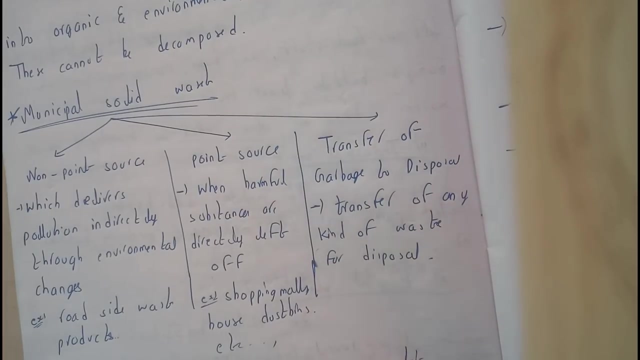 That's it. There is nothing much to think. These cannot be decomposed, So municipal solid wastes are furtherly divided into three types. One is non point source, point source, and the municipal will be transferring from garbage to this person. That's a method, but I included in the types 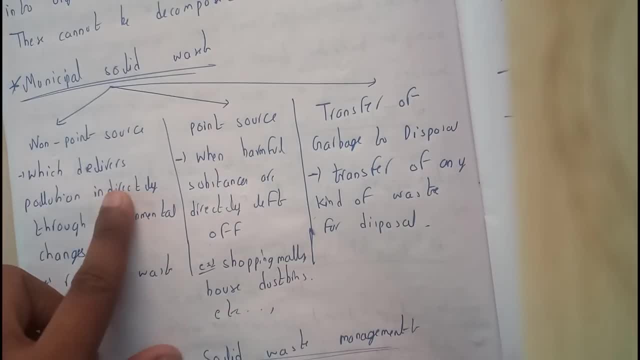 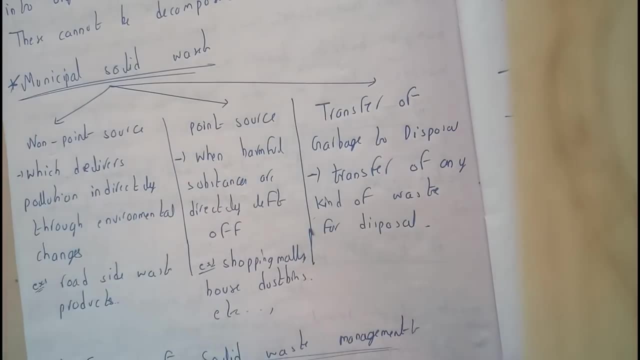 That's fine. Okay, Non point source which delivers pollution indirectly. In one of my tutorial, I have told you what is a non point. Which is indirect waste? Okay, It is a type of pollution of environment, such as roadside waste, roadside waste products. 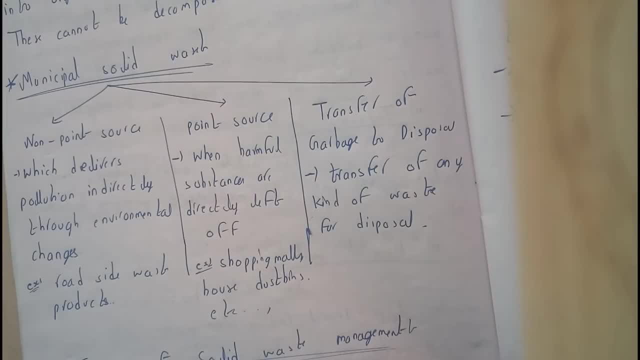 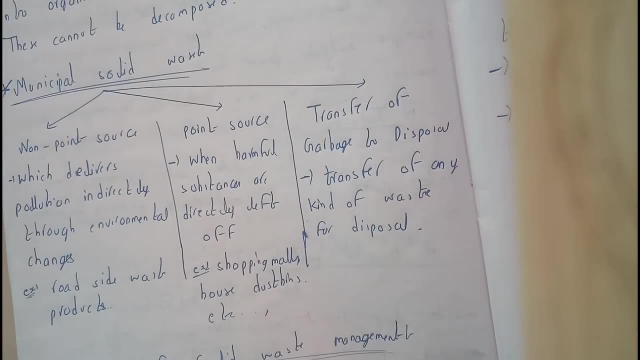 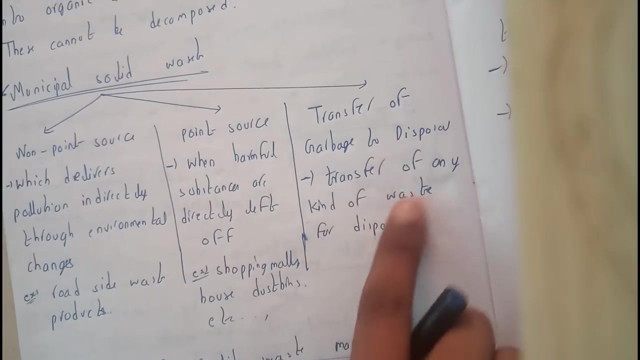 They have no use and they cannot be degradable. And next, whenever we go through point source and the harmful substances are directly left out, such as shopping malls and in household, household wastes and in our dustbins, etcetera. Transform is transferring of any kind of waste to disposal from gas. 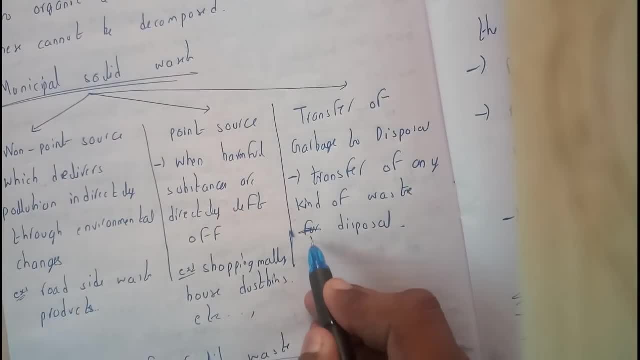 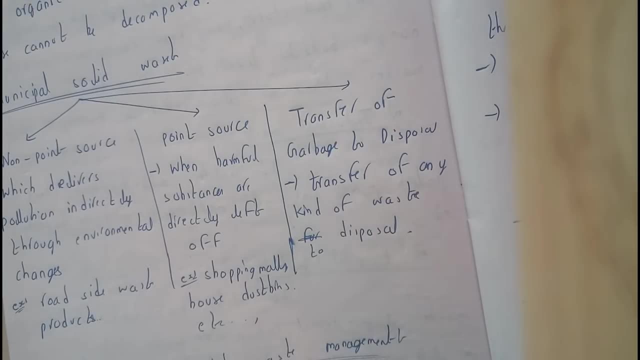 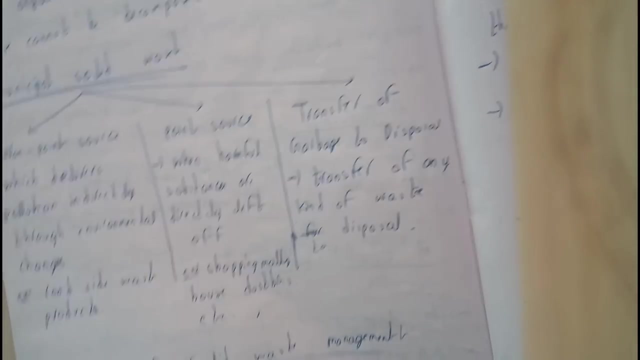 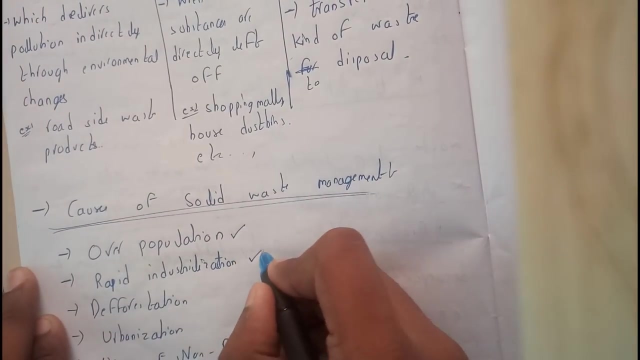 Okay, Solid waste to disposal, guys, solid waste to disposal. I hope everyone is clear now with what is municipal waste, What is municipal waste management, What are biodegradable and what are non biodegradable and types of solid wastes. And let's go through causes now. causes of solid wastes due to air pollution, rapid industrialization. 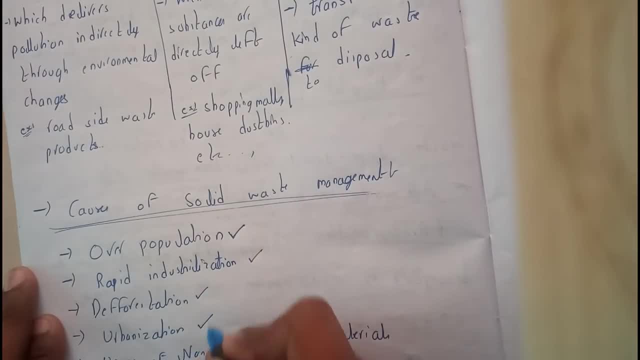 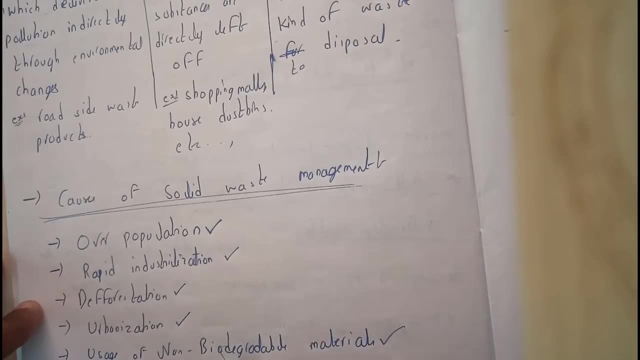 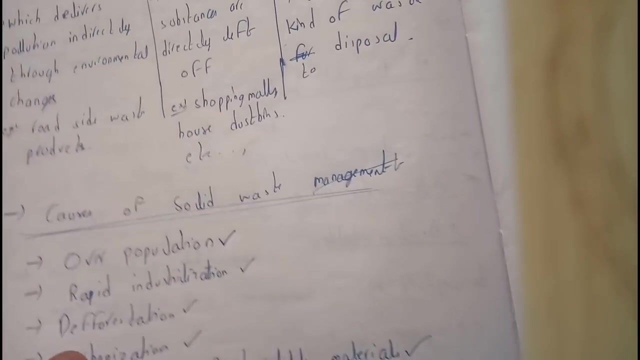 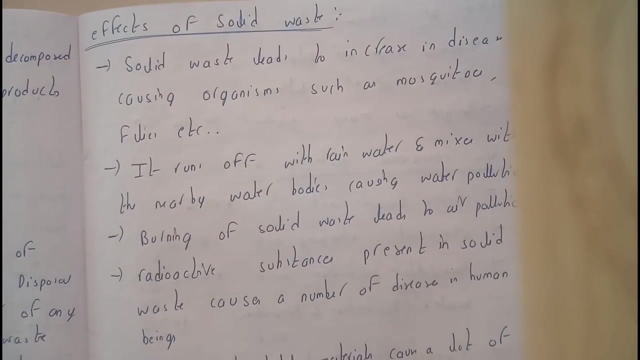 overpopulation and deforestation, Urbanization And usage of non biodegradable materials even cause solid waste. solid waste, causes of solid waste, could be better. Okay, And lack of public awareness. even that also includes in it, And let's go through effects of. I hope okay, just a second. okay, now it's clear. 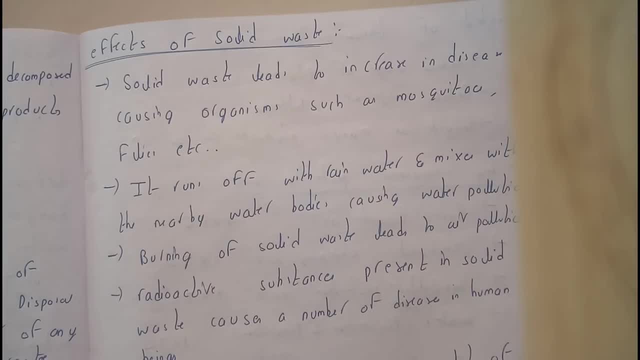 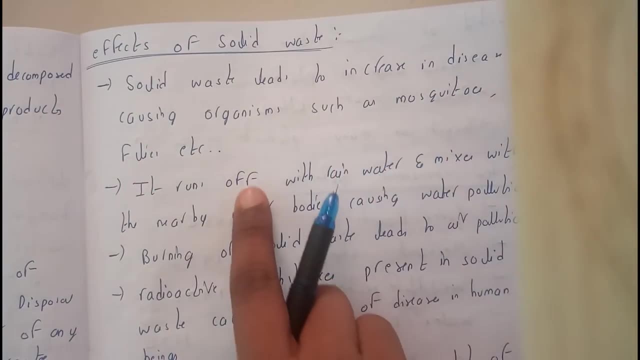 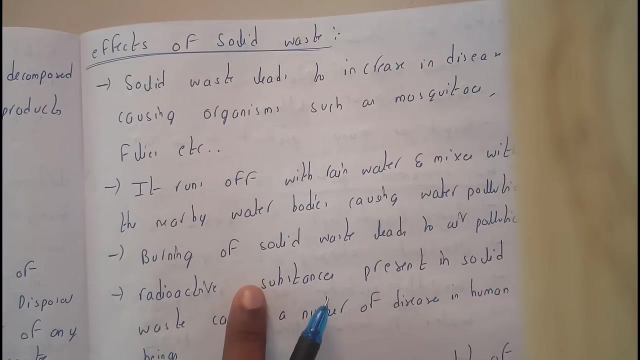 Okay, Let's go through effects of air, effects of solid waste. Solid wastes lead to increase in diseases, causing organisms such as mosquito flies. They can cause many kinds of diseases, guys: mosquitoes, malaria, dengue, etcetera. Okay, 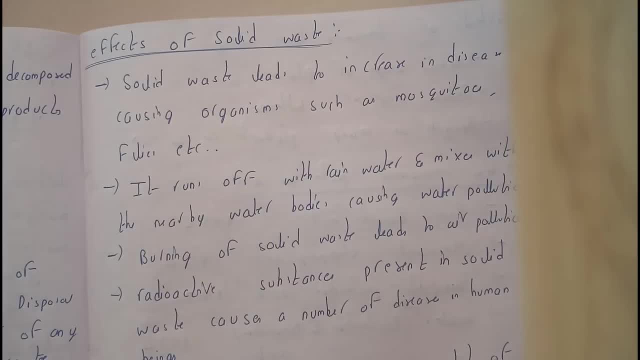 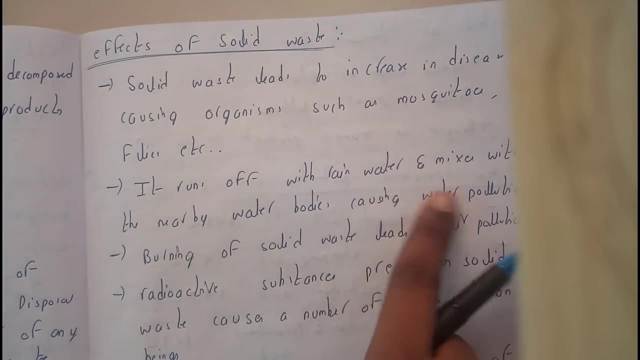 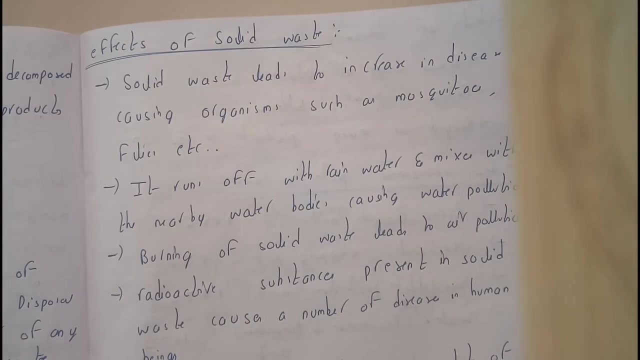 That is due to unwanted materials in our surrounding, which we can call them as solid waste, And it it runs with rainwater and mixes with nearby water bodies, causing water pollution. If they are just thrown on the road, Okay. If there is a huge rain, it moves with the water to the nearby ocean or lake or any nearby. 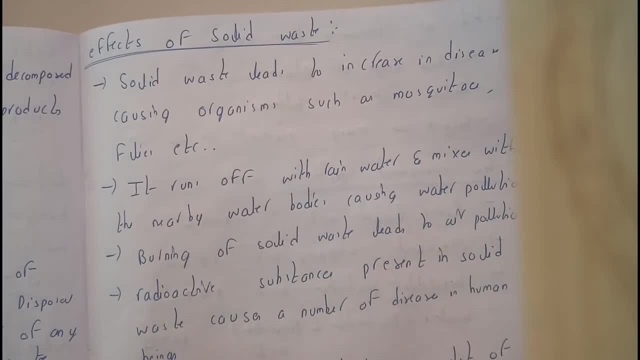 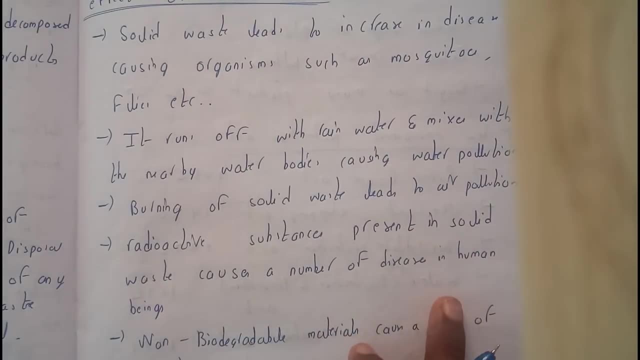 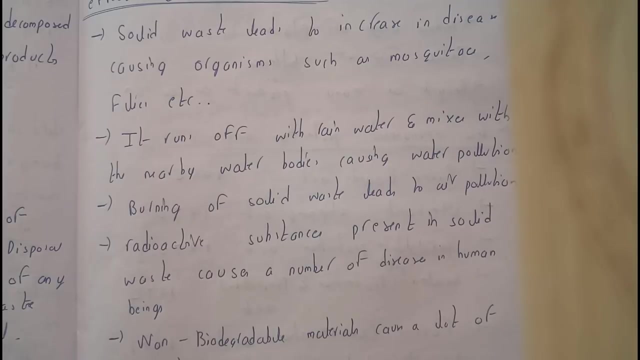 sea or ocean or somewhere, so that it causes water pollution. Even burning of solid materials lead to air pollution, and radioactive substances present in solid waste cause N number of diseases, guys, It is not one or two disease. N number of diseases which cannot be defined by a man. 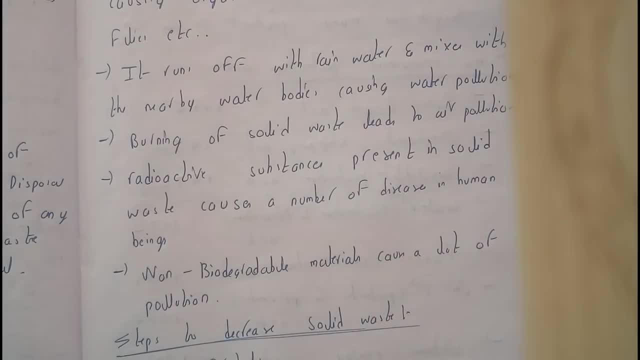 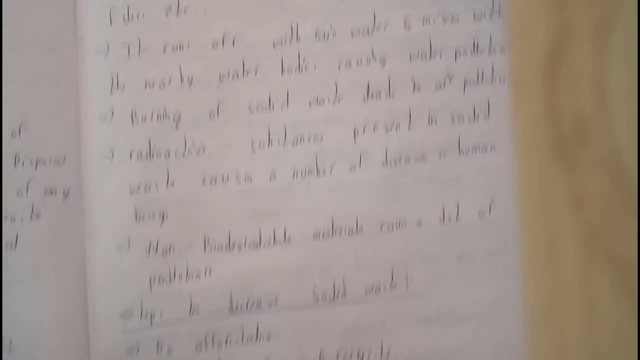 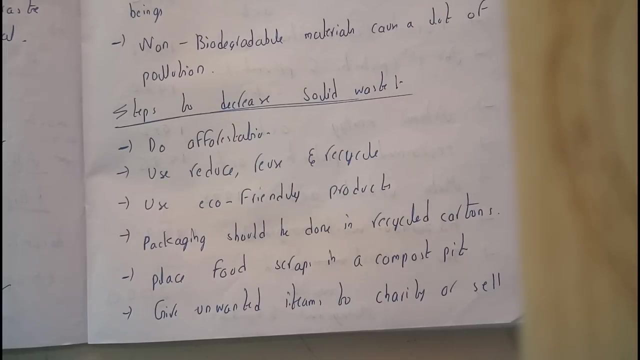 And even non biodegradable materials causes a lot of pollution, guys. So Now a bit clear with solid waste. Okay, Let's see some steps to decrease solid waste. We need to do afforestation. Use, reduce, reuse, recyclable materials. 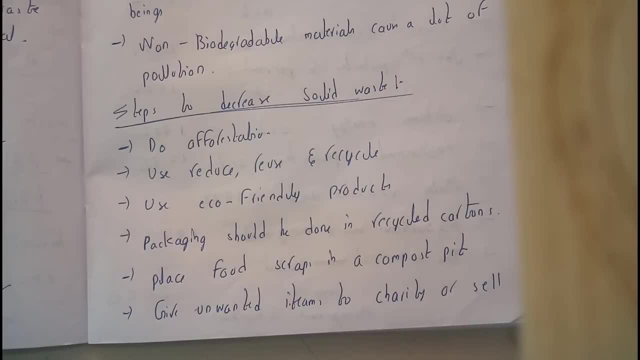 Use eco-friendly products. Package materials should be packed such that they can be recycled again, And package materials should be package will be using package bags or boxes or something. They should be made of recyclable materials. Place food. Place food scrap in compost pit.